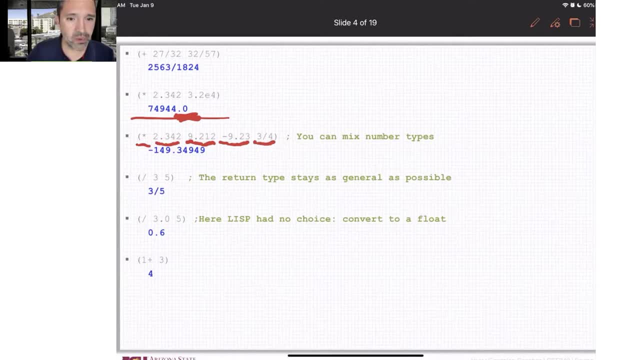 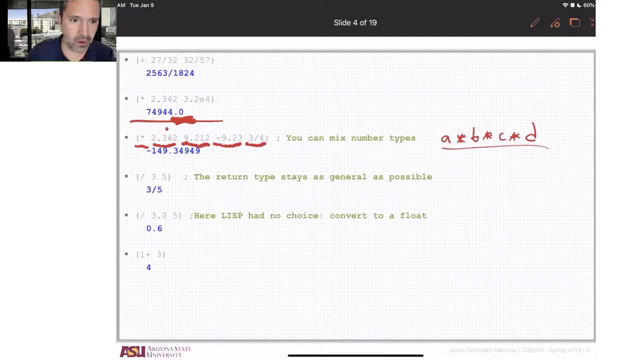 another one and one fraction. So I am doing the multiplication of four elements. So this one is something like one element, multiplication. the second one, multiplication. the next one, multiplication, the next one. You can mix: floating-point number, floating-point number negative, floating-point number one. 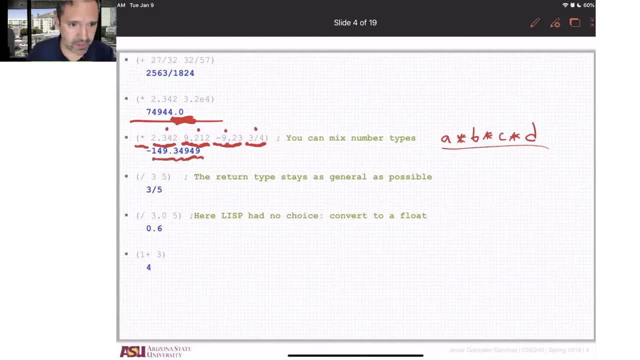 fraction. In this case, the representation that is going to be used for the final result is this floating-point number. So float, float, float, and when you multiply for the fraction, it's going to still be this float. As mentioned before, if you do the division of two integers by default- and this is a- 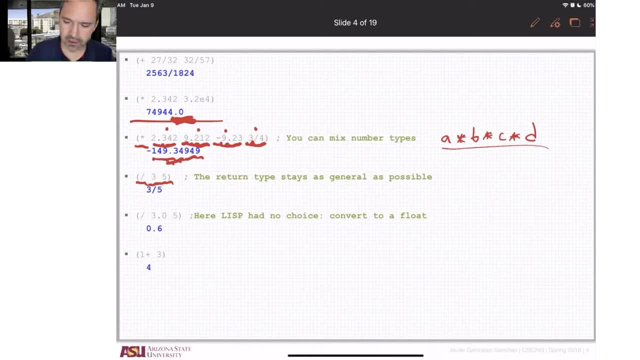 rule Lisp is going to transform your integers to a fraction. If the computer can give you the fraction, the fraction has priority over giving you something decimal. Now, if you do something like this and you involve floating-point numbers, even though you put the point zero, 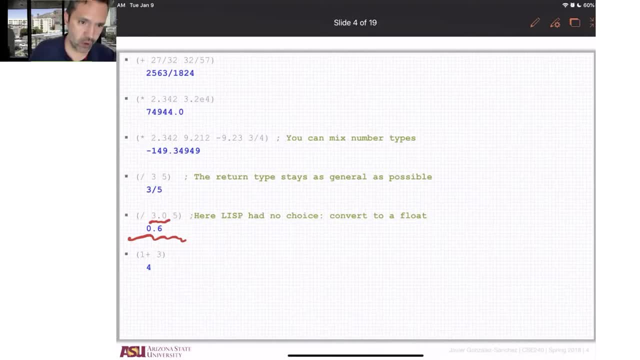 on, come up doesn't matter. but when you do a division and the division involve floating-point numbers, your result is going to be a floating-point number, This one, Parenthesis one plus three. What is the name of the function? there" Is one. 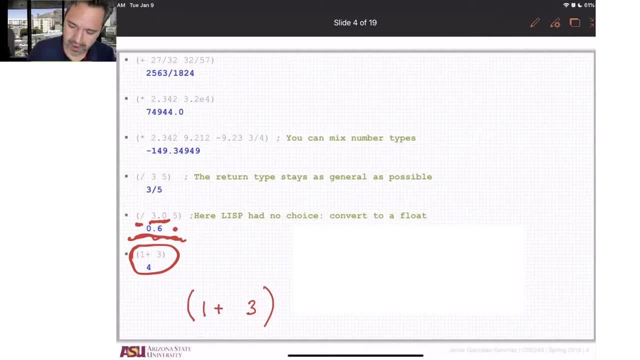 plus. Well, remember parentheses, everything until we found a white space is going to be the name of the function. so this one plus is the name of the function. what is the meaning? you can guess: the plus plus from Java, C and C++, this idea of incrementing one. 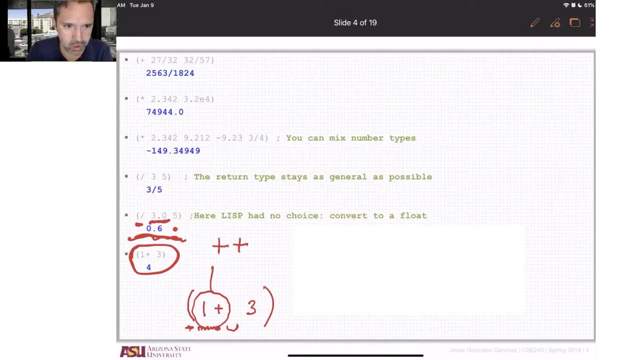 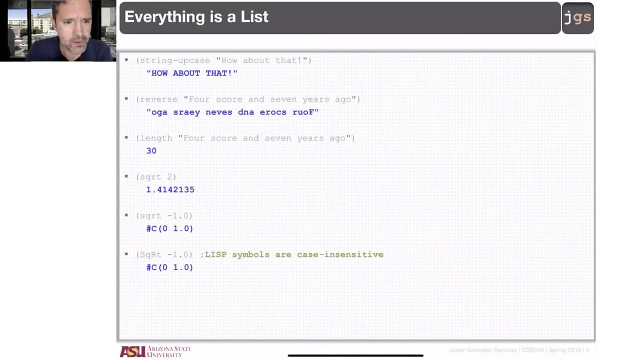 here the name is one plus and then the parameter next. obviously you have in this all the operators, or everything that you knew from Java, C and C++. there are also functions. if I show you new functions like length, reverse, string, uppercase, sqrt, whatever, 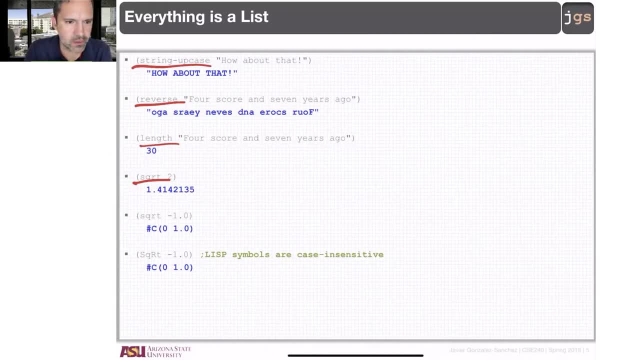 some of the functions are kind of easy to understand. you can figure out the idea with the name. One thing that is important: usually in Java, when you want to put the ID for something, what you do is these two words like string uppercase. this is Java. it is like two words together. 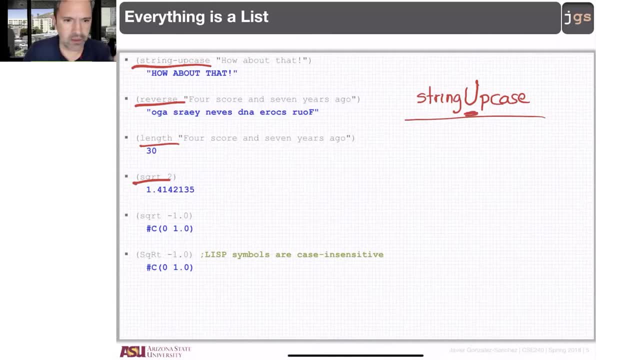 string uppercase, starting with the second word uppercase. so the reader is going to identify that there are two words. This is Java. C++ can follow the same With C. we review that the idea. with C is two words, they are separated and we use the lower underscore. So basically, 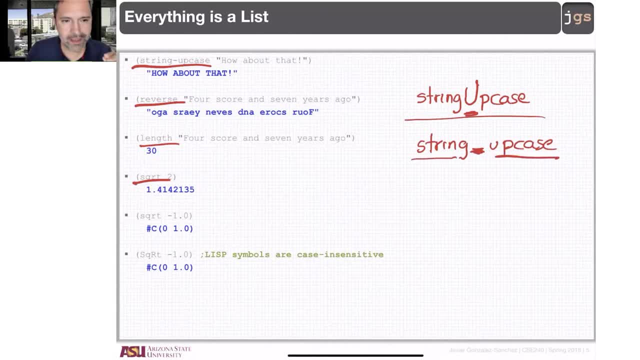 underscore one underscore word two. In Lisp, instead of using the underscore they use when you have two words, you use the minus to connect them. So for instance, this function string minus uppercase, is one name for one function. I am not doing a subtraction there. 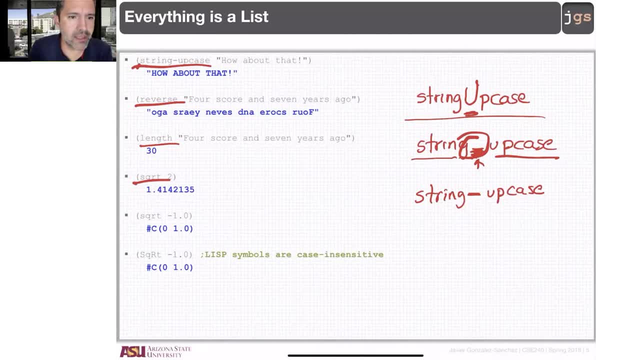 We put this line. We put this line there connecting words. It's one more character that is part of the name of the function. So in this example, my function name is string minus uppercase. That is the full name for the function And we have only one parameter. That parameter is a string. 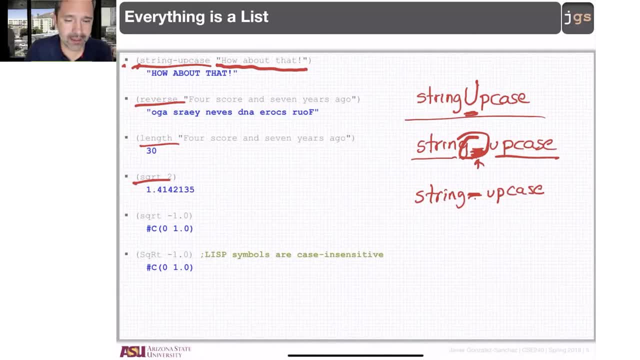 And you can figure out the function. string uppercase is basically a function that is going to return the same string that you put there. So this function does a parameter, but every single character in uppercase And obviously for the symbols. well, they are going to return the same, Only uppercase for the letters. 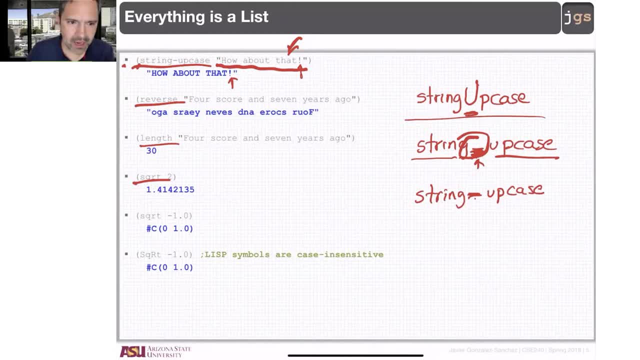 right For the alphabetical characters, Similar. there is a function reverse And this function reverse receives one parameter and basically returns the string in the opposite order. So you can notice, the first character here is, the last one here, The second one is here and so on. So this one goes there and this one goes in this direction. 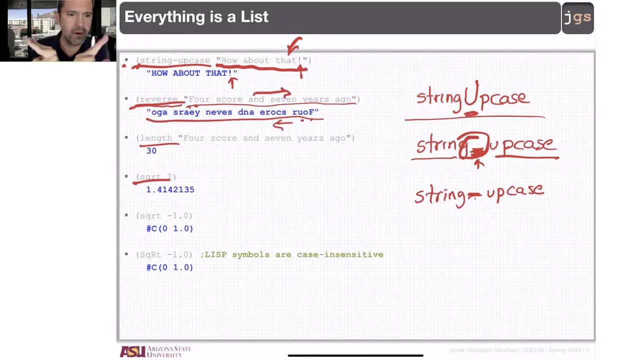 It's just take all the characters and reverse the order. Length is how many characters do we have in the string? So basically it's counting how many characters there are and it's going to return a number Square root. We mentioned this before. 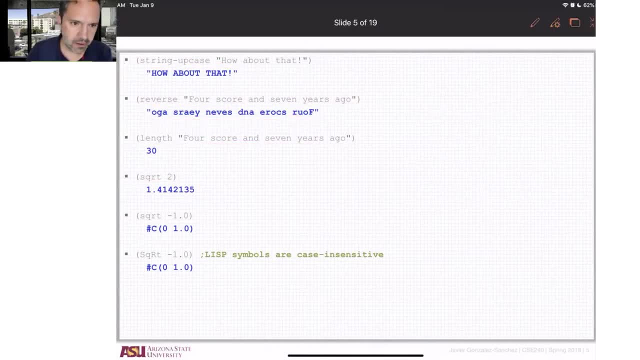 Square root And you can use an integer, An integer number, And the result is going to be a floating point number, as you can expect. And you can use a square root, a negative input, and the result is going to be a complex. 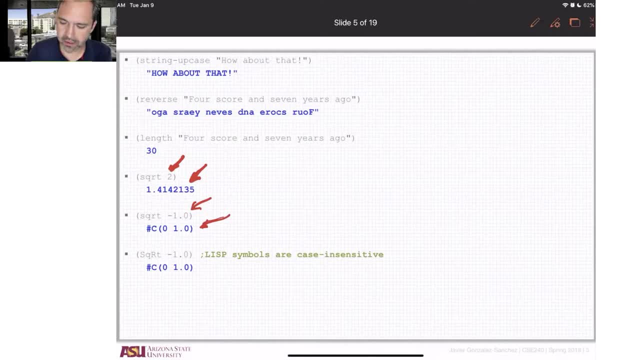 number. And remember, this is your complex number, real part, imaginary part. So square root of minus one is one, i. You can use the name of the functions, as we mentioned before: Lowercase, uppercase, or a crazy combination of upper and lower cases, like this one. 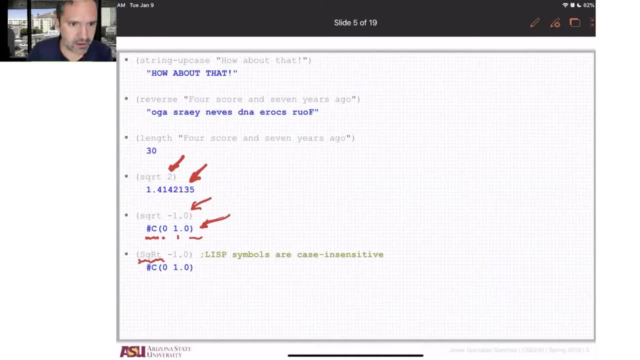 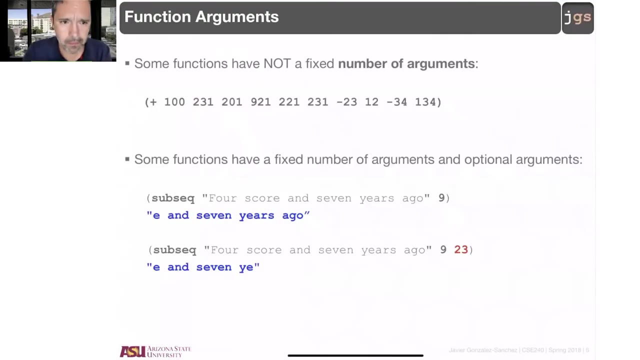 This sqrt with the s in uppercase and the r in uppercase is exactly the same as this one. So this one and this one are the same. So the result is the same. And again a comment semicolon. Now, basically, most of the functions do not have a limit of. 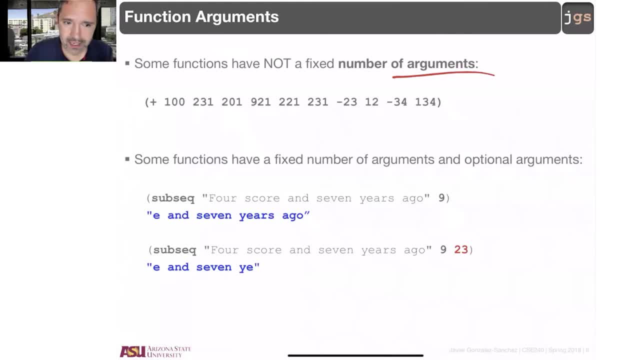 Parameters, Arguments. Basically, for instance, if you do a plus, you can call the plus with two numbers, or you can call the plus with a lot of numbers. Moreover, you can call the plus with integers or you can call the plus using fractions. 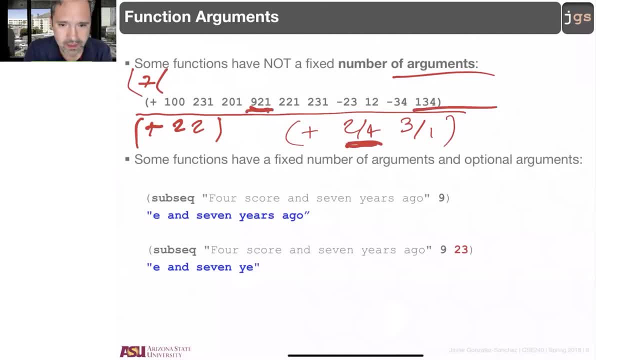 And all of the different combinations work. Moreover, some functions like this one are going to work just like overloaded functions. in Java, You have the function subseq. This one, This one in particular, received two parameters. Number one is a string and the second one is a number, and you can figure out what is. 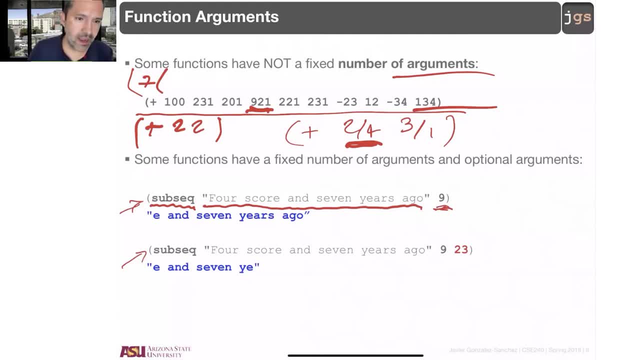 happening. Basically, subseq returns a substring. if you remember substring in Java and that substring is basically starting in the character nine to the end return. So return all the characters in the original string Starting in the number nine. Return all the characters in the original string. 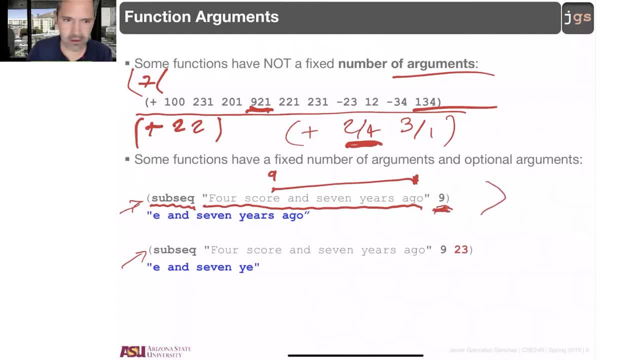 And this is the way you can add the number nine to the end. But you can also call the same function, instead of with two, with three arguments. I add one more here and is the same name, the same function, but now with three arguments. 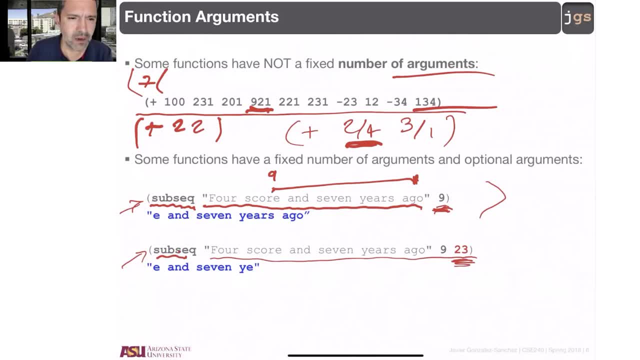 instead of two, And in this particular case, well, the nine is going to be kind of the beginning of the string, end. the second number is going to define like: okay, that is the end. So give me all the characters in the string between 9 and 23.. Now, very particular thing, I 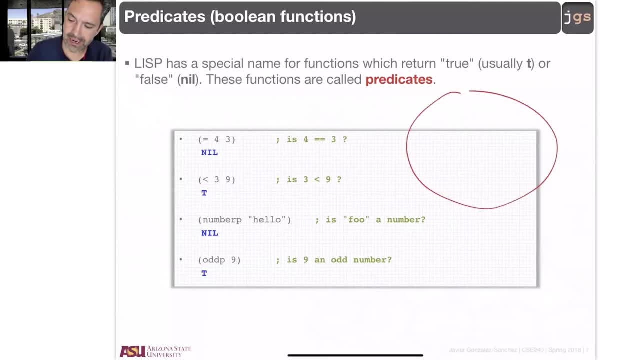 mentioned that we have list in Lisp. Anything inside of parentheses is a list. Then I told you that we have functions. Functions are lists when this one is a function ID. Well, now I need to introduce a particular type of function that we're. 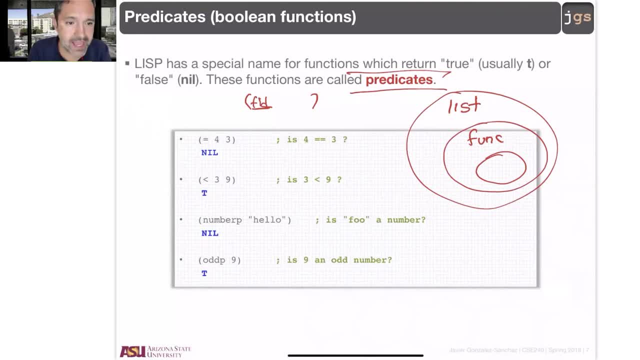 going to call predicates. A predicate is a function that returns t or a function. t or nil is a function that returns a boolean value. So any function that returns a value one of these two is a predicate. So list function: predicates. Any predicate is a function. 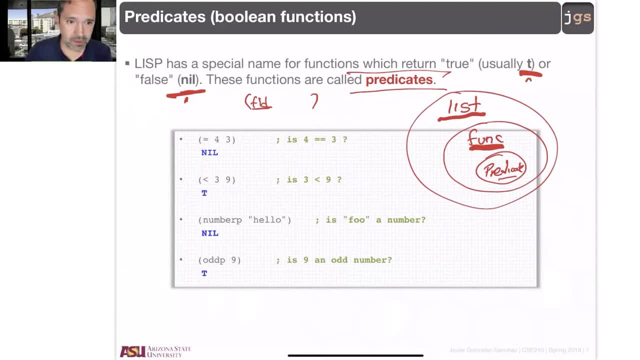 Any function is a list Examples. This one is a list Parentheses. parentheses, three elements, But the first element is the name of a function: The equal symbol. The equal symbol represents- this is very, very important one. equal in Lisp is the equivalent of the two equals in Java, C and C++. This 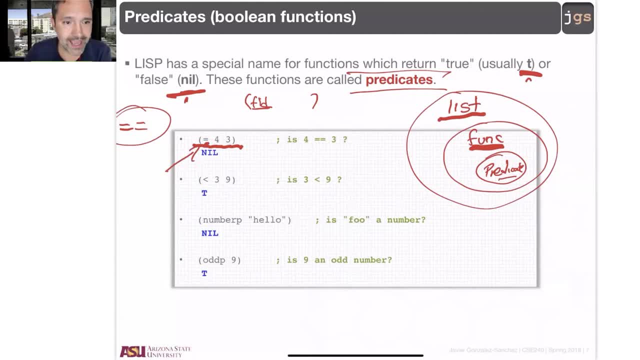 guy here is not an assignation. That guy is the relational operator equal. So this is a predicate. The result is going to be to compare if the two parameters are equal, yes or no, So something like this. in the previous languages The result is going to be t or nil. Remember there? 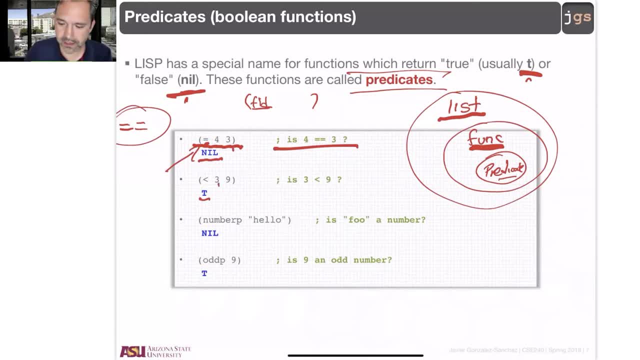 is no difference between uppercase or lowercase. So, for instance, four equal three is going to tell you no. The value for that negative value in Lisp is nil, And this is a predicate because it's a function that is returning nil or t, In this case nil. I used this one. 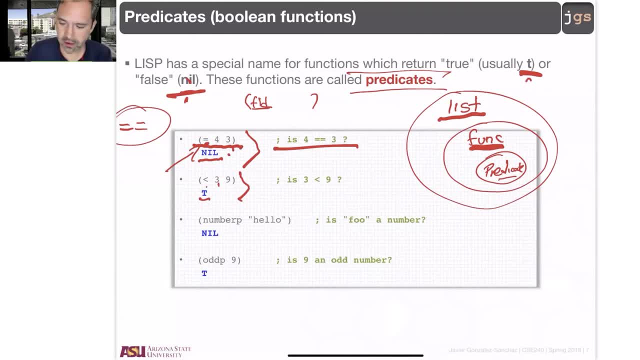 before Lower than two values is going to return, whether or not the three is lower than the nine. In this case, true, So it's going to return t uppercase. I think these two examples are kind of equivalent to something that you already knew, and I showed you this. 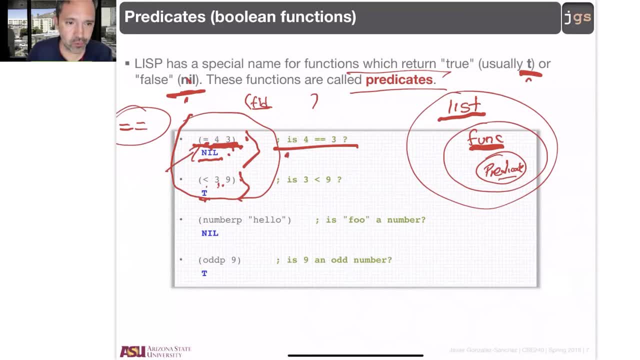 before Now, Particular names for functions. This one, Every single time that the name of a function ends with the letter p, whatever. If you have a name like here- number- I do not know what number is going to do- But if you have the letter p at the end to tell you that this 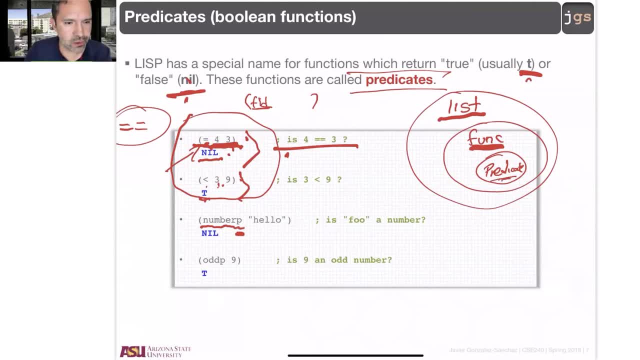 is the name of a predicate, That this function is going to return t, True or false. So this number p returns true if the argument is a number whatever, a number in whatever format, and it's going to return nil if you use here any other thing. So for: 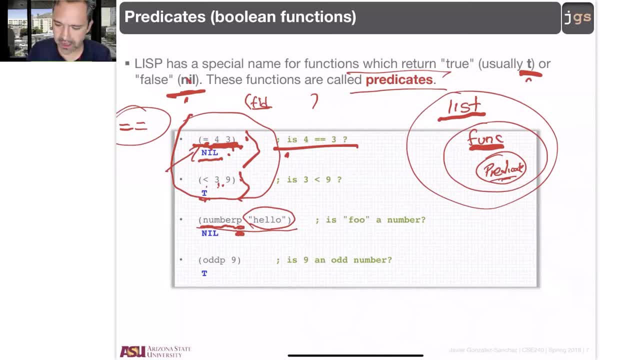 instance, number p is asking if hello, with the quotation marks, is a number and of you leave not a number because it's a string. so you're going to have nil as a result. Similar with this one. or ddp, we have the P. This one is a predicate, so it's going to tell me true or false. 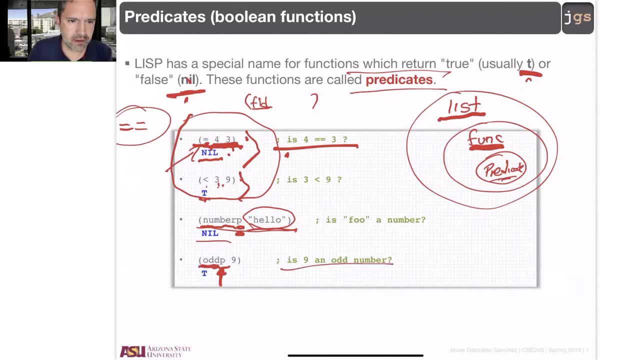 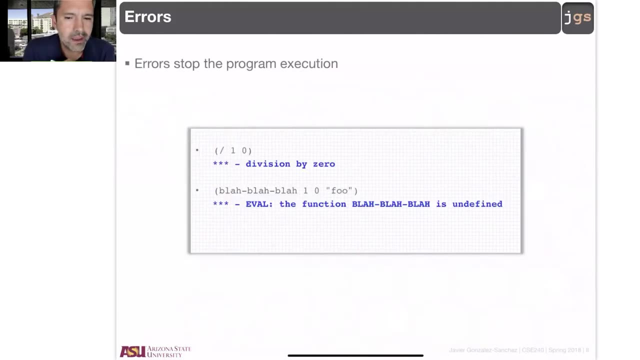 nil or T. The number is odd, yes or no. I put a number there. It's going to tell me yes, T, or it's going to tell me nil. So predicates nil and T Errors that you are going to receive in Lisp. The most common error is related with parentheses. 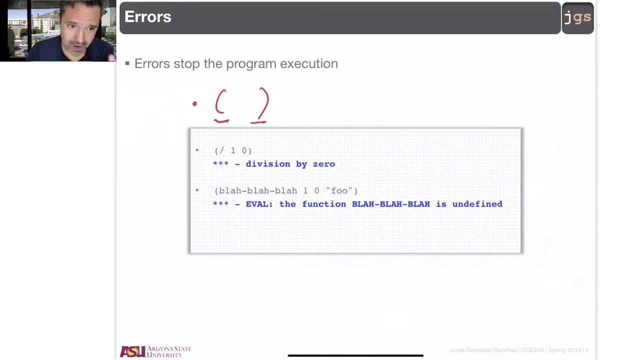 You open more or close more, whatever. Outside of that, in runtime, when you are done with parentheses, two things could happen. Number one: division by zero. Division by zero is an error. It's a runtime error, So we do not handle the. 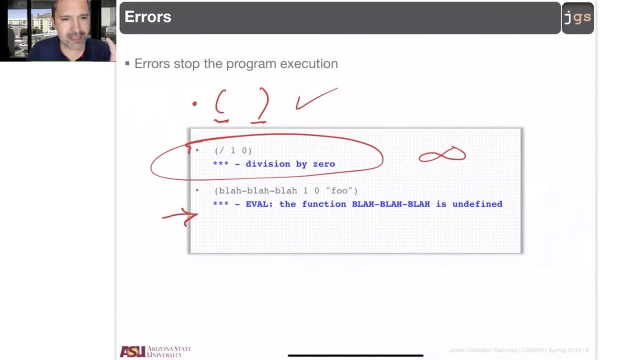 infinite values. The second thing that can go wrong is that we don't know the infinite values. The second thing that can go wrong when you call a function is trying to call a function that do not exist. So imagine that I put this- open parentheses, closing parentheses- and I put here a name, my name, and I put: 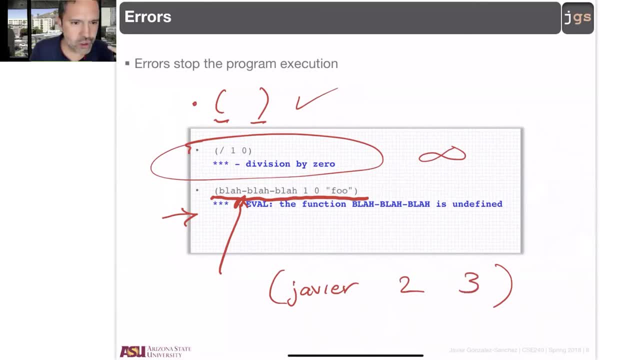 parameters. If I give this instruction to Lisp or this instruction, this is the error that you are going to receive. Basically, it's going to tell you: hey, you are calling this function because, remember, this one is the name of the function and that function. 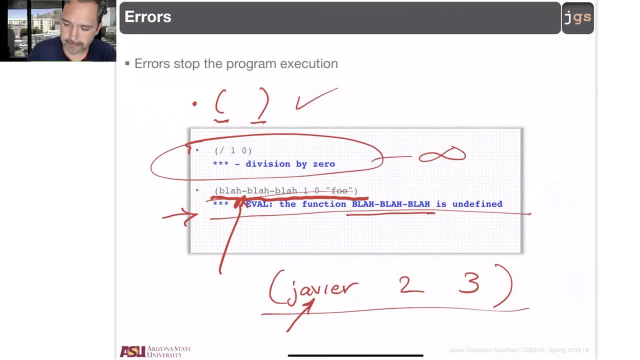 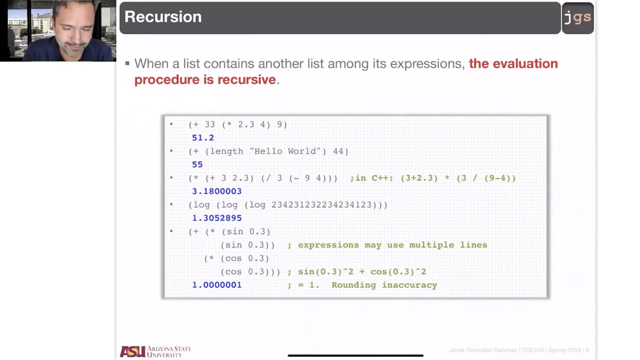 do not exist. Division by zero, undefined functions and parentheses- These two runtime error. This one is going to be basically a syntactical error. Recursion: One of the most important characteristics in Lisp is the ability to use recursion. Every function in Lisp can be recursive. Any function can be The way. 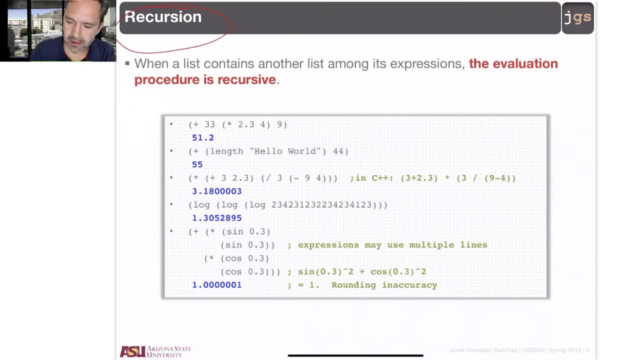 that you create a program in Lisp is putting together parentheses And, as you know, the parentheses inside are going to be executed first, The parentheses outside at the end. Your program is going to be a combination of things inside of parentheses, All of these. 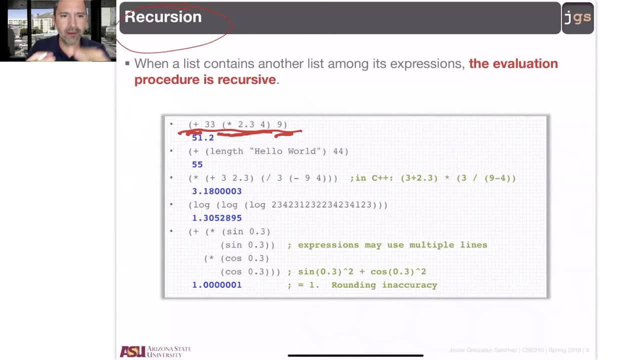 examples are one line, but we're going to start working with programs that use seven lines. But you need to remember if you open a parentheses, that parentheses should close in some point. Lisp don't care if you use the enter or not. Usually what we're going. 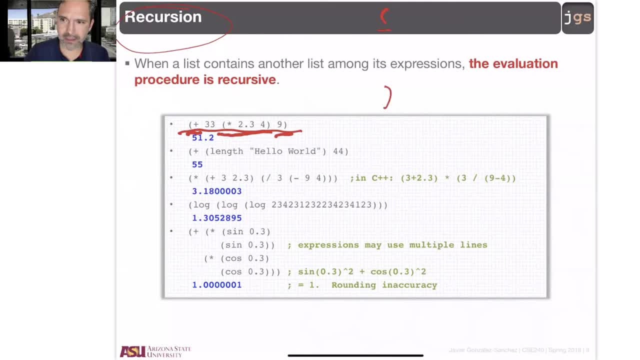 to do is open the parentheses here and maybe close the parentheses here, and in this Hm part we're going to have a program and that program is going to be more parentheses, maybe outside or maybe with things inside, But again, open, open, open. 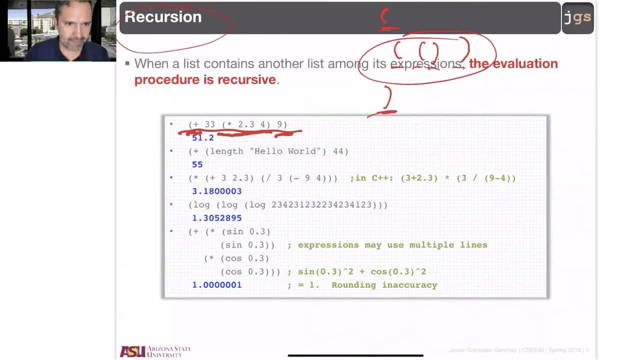 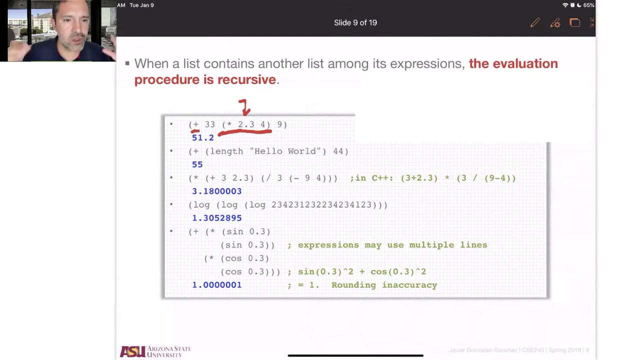 close, close, close. they match. the program is correct. So the idea here is: whatever you do inside is executed first. So for instance, here I do the multiplication first and whatever is the result, of the multiplication is going to be a parameter for the addition When you put a parenthesis inside of. 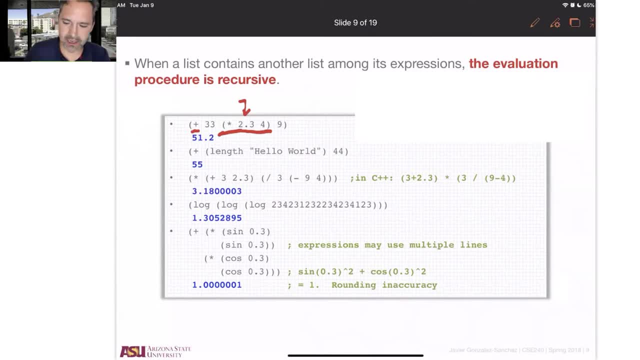 another parenthesis. basically, the meaning is you have a function calling another function every single time. This parenthesis inside of parenthesis is calling a function and the first function, the one that is outside, is called a function. It's going to be like the main in your program, So you start with the plus that. 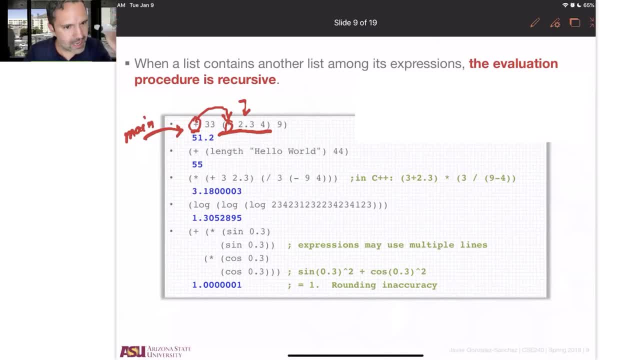 is the one that you call first, but then the call inside has the multiplication or whatever, and it's like the plus is calling that function and when this function finishes, whatever that function returns, the plus is going to use it. This is basically the result of 2.3 multiplication 4.. 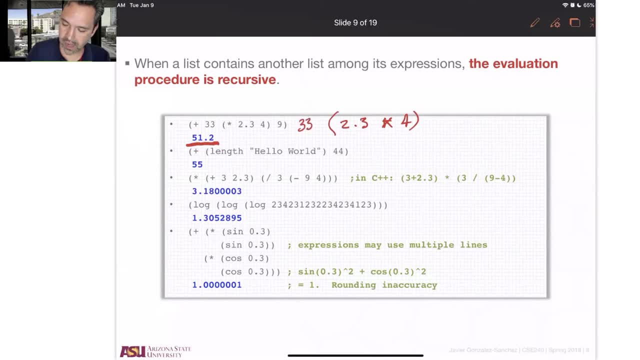 So it gets an addition, but it's very difficult and laborious, so I want that. I like to talk about other things, like going downstairs, For instance. all three of us can go downstairs And I don't belong here. 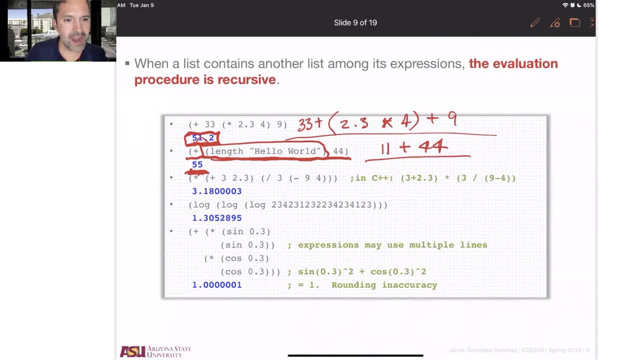 So I do incomplete. So I go inside of a building and I go outside The figure, there is the next thing And then I also do the multiplication and then I do multiplication. result that you saw on the screen is the result of the last operation And things. 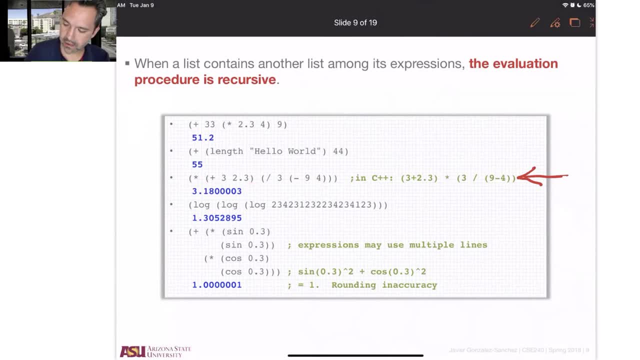 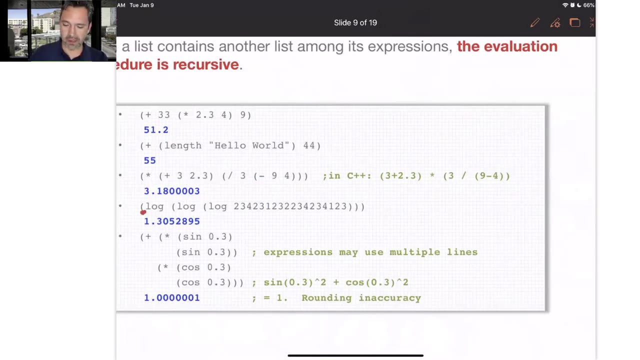 can go crazy. Can we understand that this one is basically this operation here? I am sure that you want to use maybe this one or maybe this one or maybe this one For the mathematical operations, at least the common ones, if you remember the name. 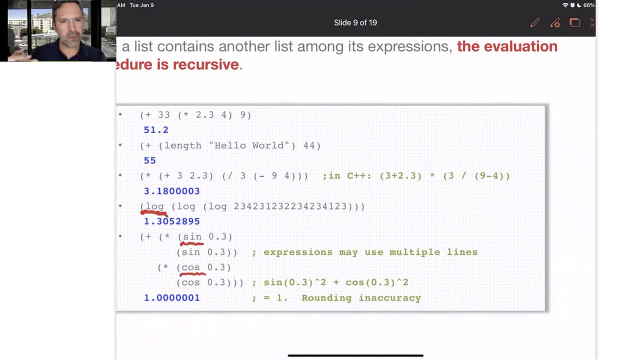 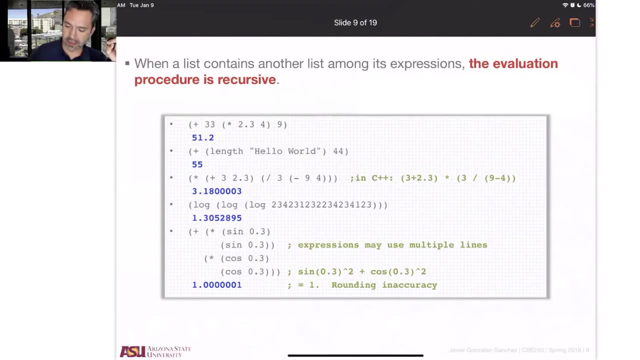 in the Java libraries. those are the same names that you have in the math library for C, C++, And it's going to be almost the same for the functions ID in Lisp. This one is a very common problem. Okay, What I am doing there is this one: The multiplication to do the pow2 and the addition Result. 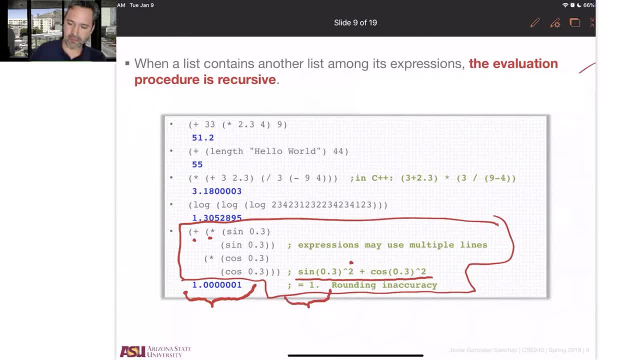 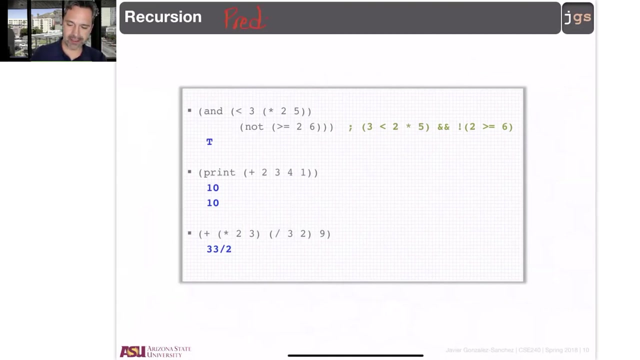 Result: Nothing is perfect. You notice, here we have this ghost Decimal value. Be sure that you are understanding what is happening. Practice Now moving forward. Exactly the same can happen with predicates. Remember these things that return: yes, no, true, false, T, nil. If you remember your operator, you remember those. 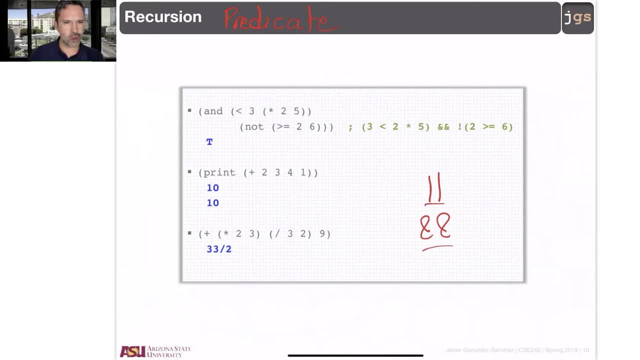 guys, Java, C++. Okay, What if I told you that, instead of using this, now, this is the predictor an. What about? instead of this guy? Not So an or not, That thing is basically this: It's a combination. 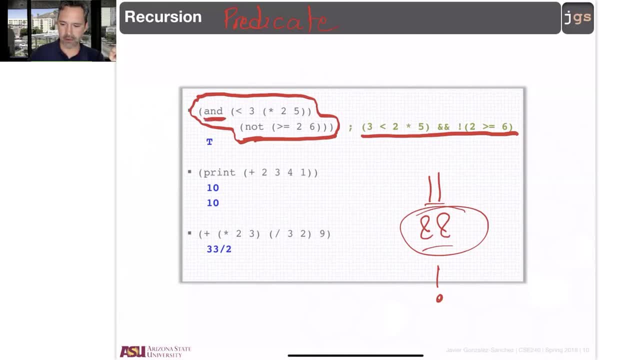 of logic operations. Okay, Arithmetic operators. Relational operators: Yes, you have greater than or equal than Use two characters is the name of the new function, And I have arithmetic operators here. This box is the same than this one, And here I put the parentheses just to be sure that. 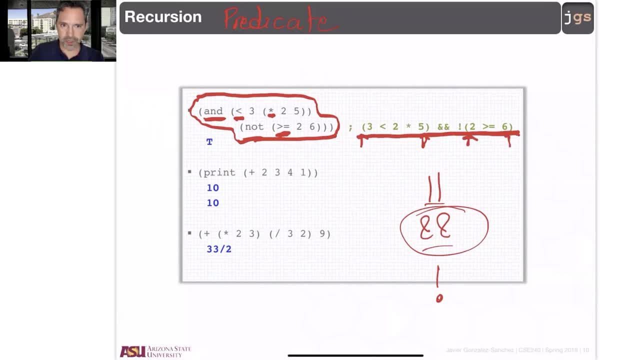 we understand what is happening first. So, for instance, we understand that this no apply to whatever is the result of two greater than or equal than six. This no, the parameter for that no is whatever is the result of this parenthesis, that is basically this: greater. 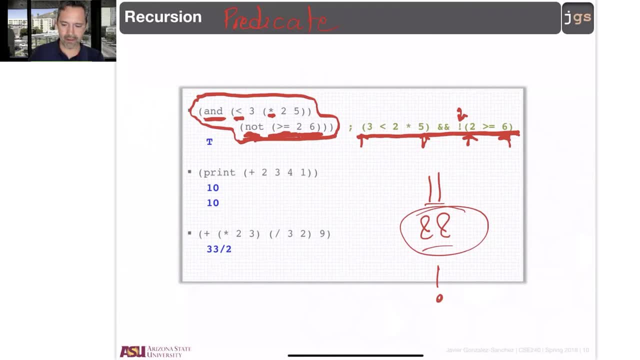 equal between the two and the six. So far, good. You notice, for the first time I use two lines, Remember: if you want to print something on the screen, there is an instruction: print. If you are using the online virtual machine, you have two columns: one with your program, the other with your output. 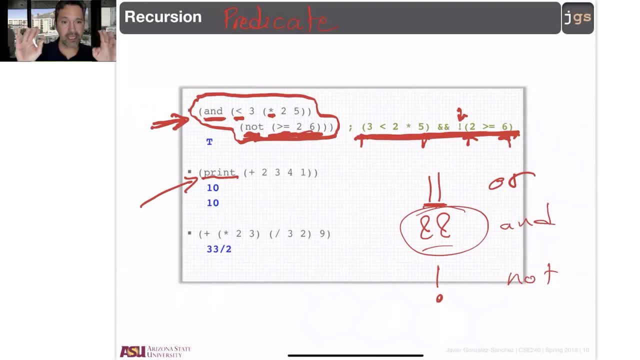 If you want to print something here, you need to use the instruction print. If you are using the virtual machine, that is local in your desktop. the virtual machine is always printing the results. But if you use print, what you're going to get is twice the value One because 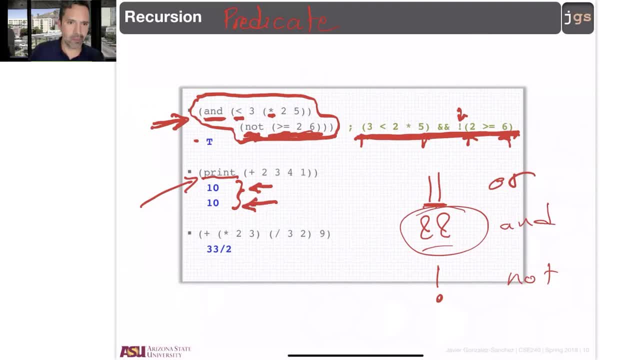 it prints the result and the other because it's the return value of the function. When you are doing a program and your program needs to print a final result, use the print instruction And it's better to have the result twice than nothing. Good, 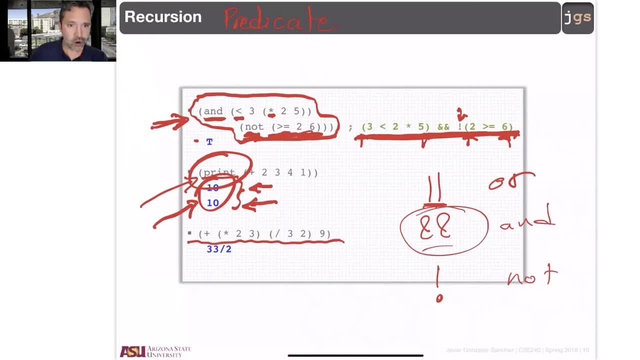 Now, this one is a big operation and you're going to notice that, for this case and several others, the virtual machine is going to have as a priority giving you a fraction number, like in this case. the result is 33 divided by two, instead of giving you floating point. 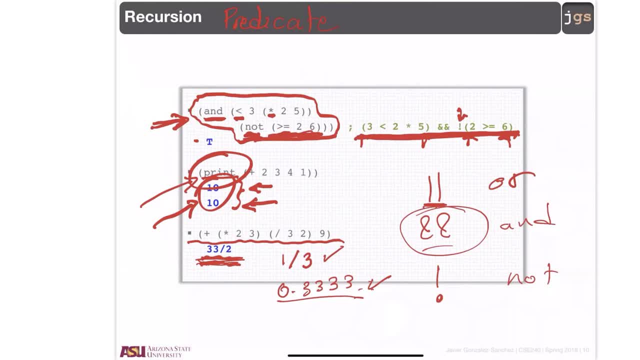 numbers. Good, Okay, guys. see you next lecture. Thank you.